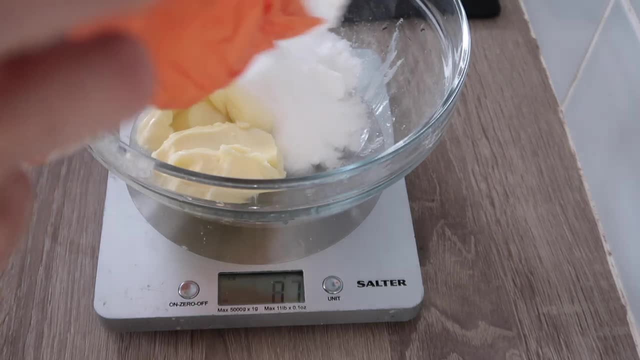 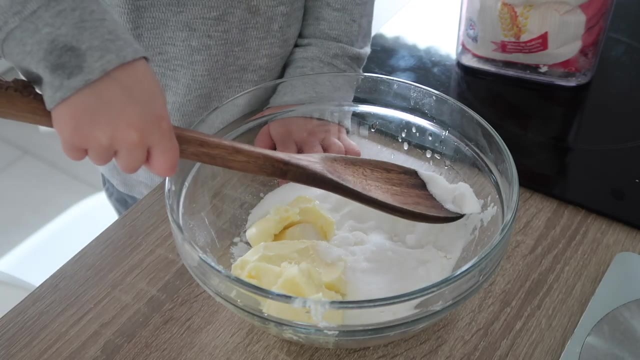 And then we're going to add in the sugar and mix these up to make a very nice creamy mixture. This is where Oliver comes in. I love to just give him a wooden spoon and a bowl of anything, and he will mix it up for ages. 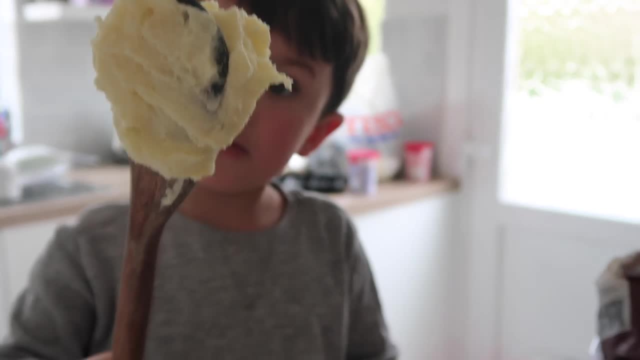 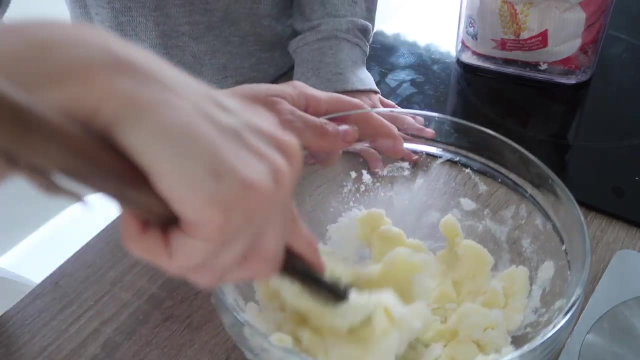 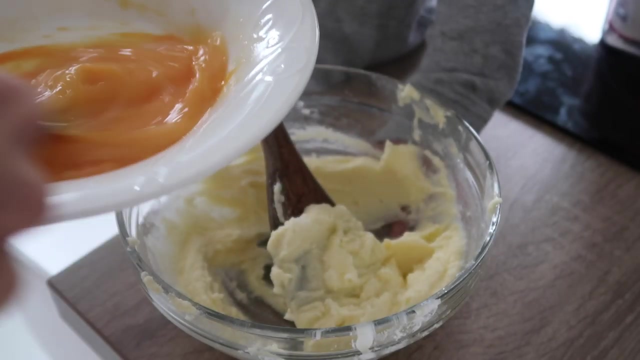 He absolutely loves to do this, And then I just need to make sure that I take my turn at the end so that I can make sure that it's all mixed thoroughly. And then we're just going to whisk up the eggs Separately, just to break them up, and then add them bit by bit into the mixture, just to make sure they're all mixing in properly. 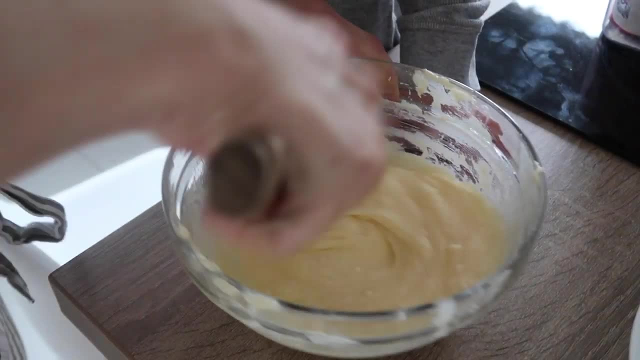 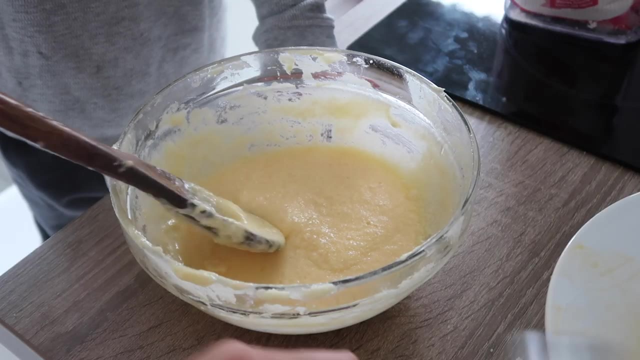 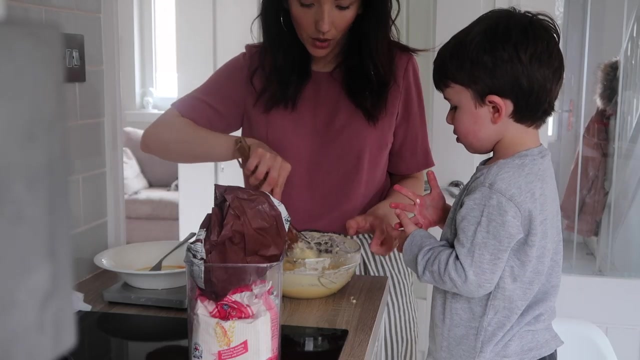 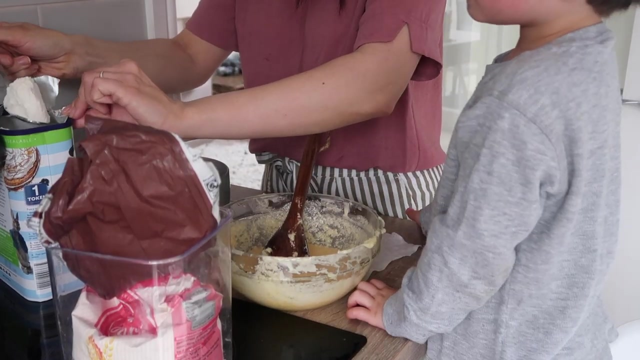 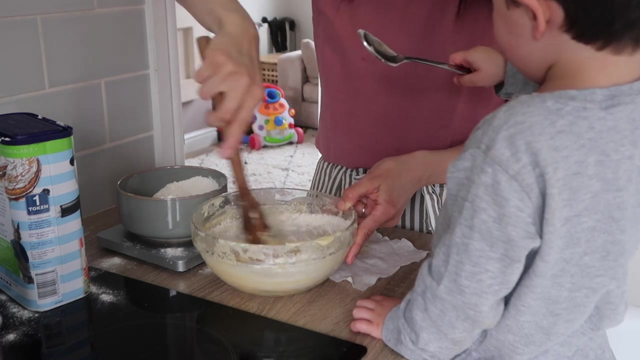 How many times am I going to say mix in this video? And then it's a teaspoon of vanilla extract, And then I'm just measuring out the flour and putting that into a separate bowl so that Oliver can add that in himself. I'm just trying to make this as smooth a process as possible when kids are involved. 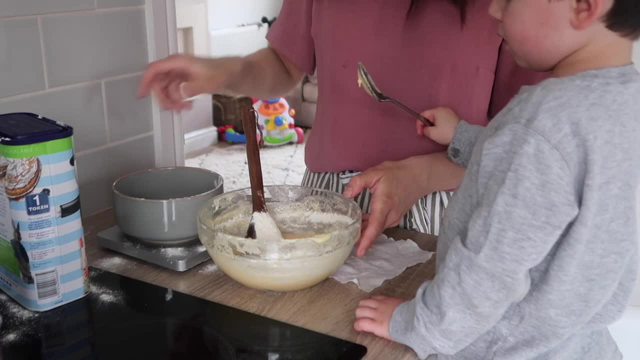 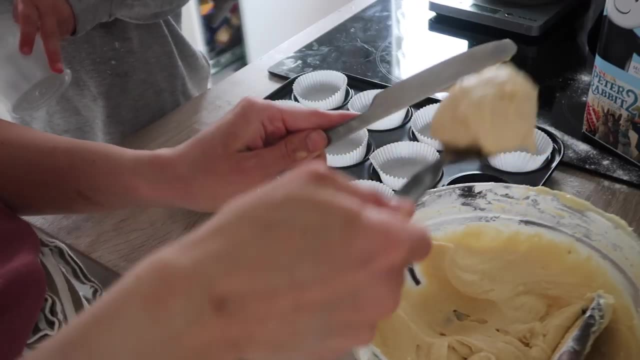 because Oliver does like to be the one that's adding things in himself and he doesn't like to get much help. And then we're just putting the mixture into the cupcake cases. Ideally we would have had 12, but we actually only had 10 left. 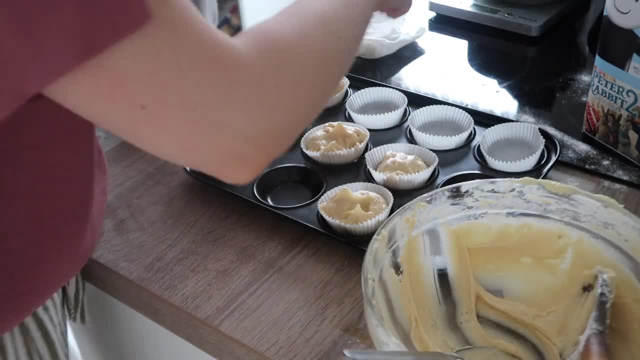 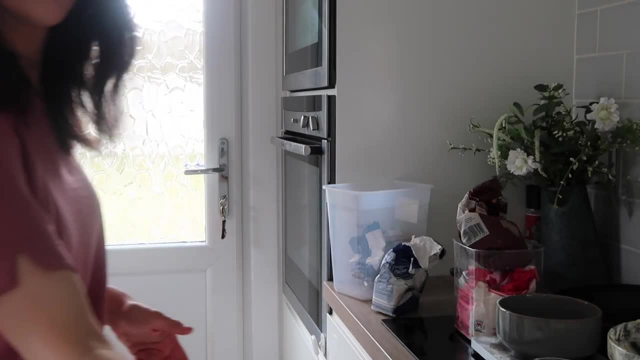 To do this, so I've kind of overfilled a couple of them, which doesn't work out at the end. But yeah, you just need to use one tablespoon per cupcake case And then you want to pop them into the oven at 160 degrees for a fan oven or 180 for a normal one. 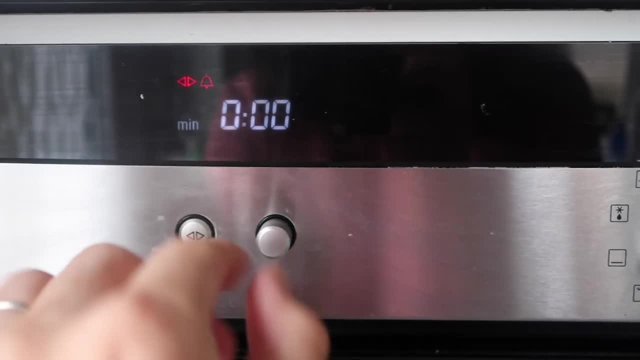 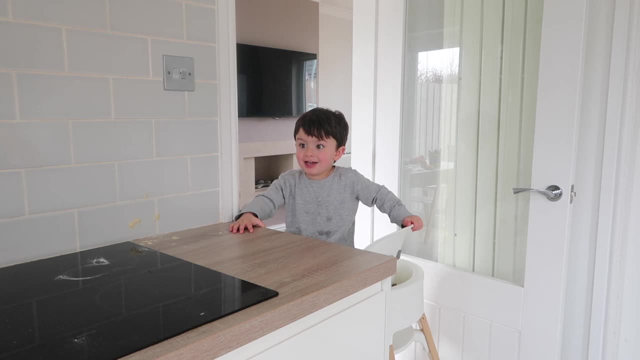 And they will be in between 10 and 15 minutes. So I've got a fan oven and it took about 12 minutes for mine to be ready. And this is my favourite part Once we've made something, it is watching Oliver's face. 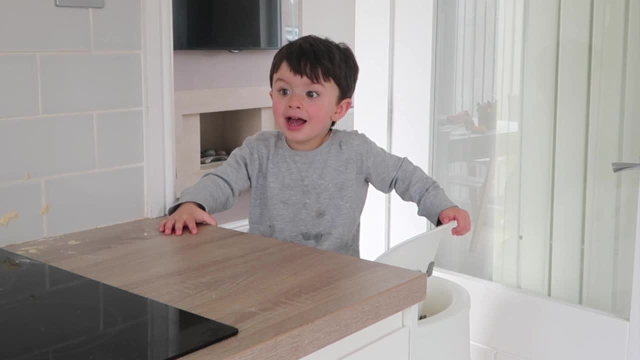 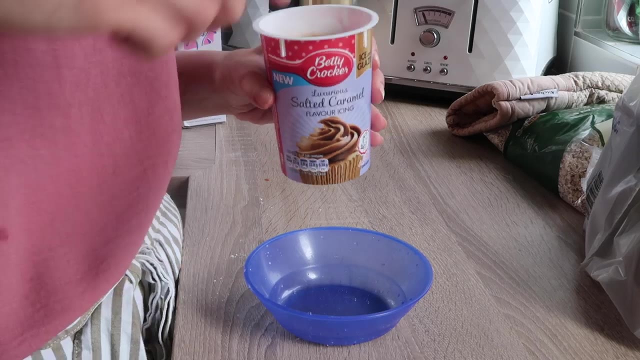 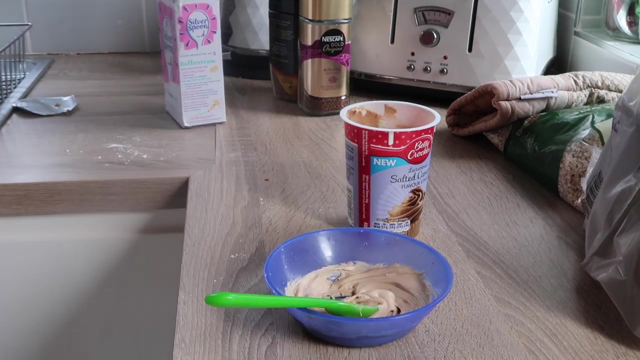 His reaction to seeing them come out of the oven. It's the cutest thing ever. And then this is the fun part. So I'm going to be using the Betty Crocker salted caramel icing. So this one's already pre-made and you just mix it up in a bowl. 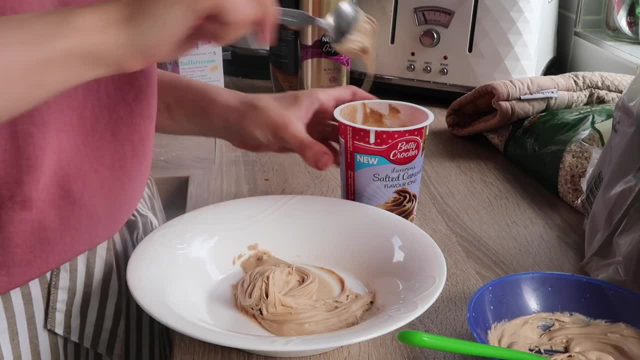 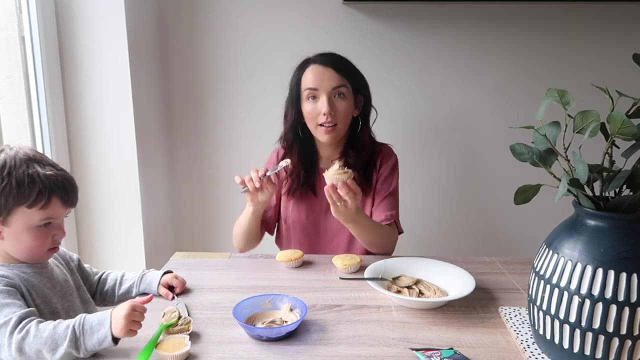 And you can also heat it up in the microwave and, like, drip it over and try and make his own little creations. These are definitely not Pinterest style cakes if you let your kids decorate them, but that is the fun for them, And we added some chocolate. 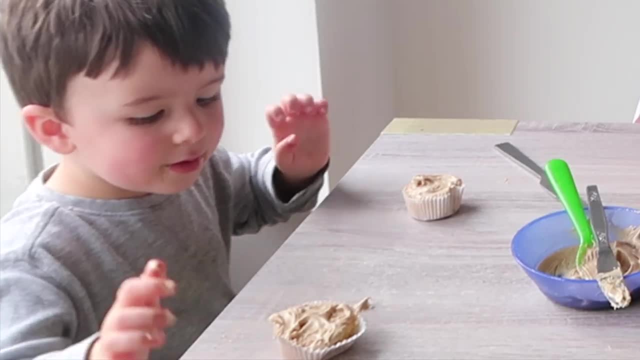 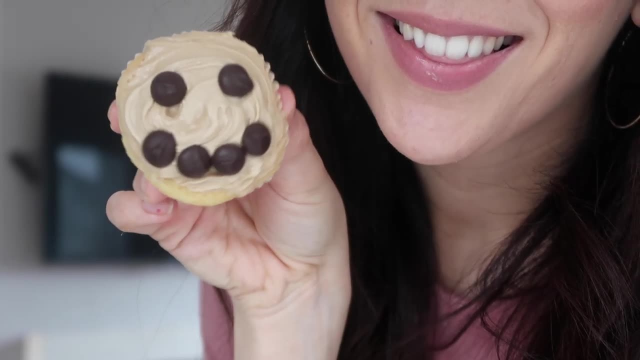 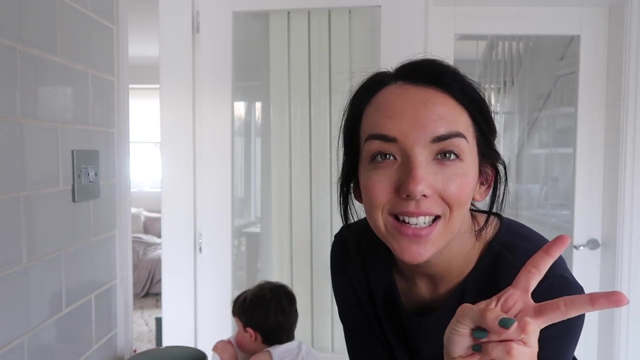 Chips on top as well And made some smiley faces, And it was actually a really fun little afternoon decorating the cakes, And he was so proud to show them off to his dad as well. Okay, so it's day two, And our second recipe that we are going to make is oatmeal and raisin cookies. 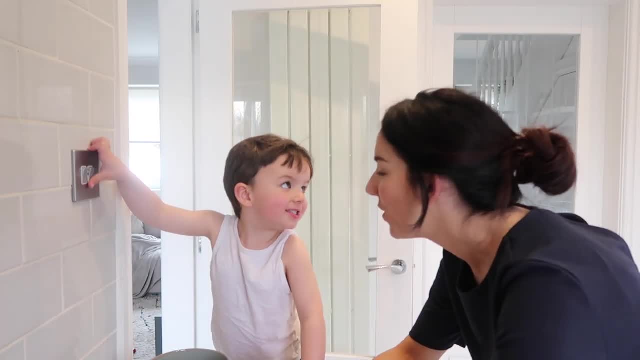 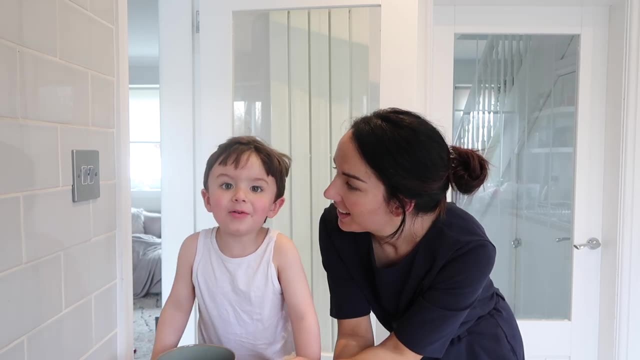 Let's get making some CAKES. No cookies. Today we're going to make some. Today we're going to make Apples. No Cakes. Cakes, It's not cakes, it's cookies, Cookies. 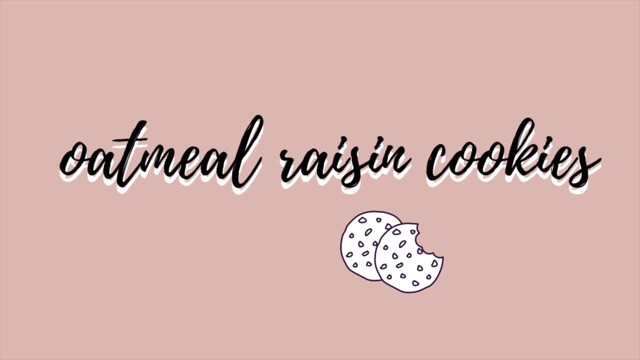 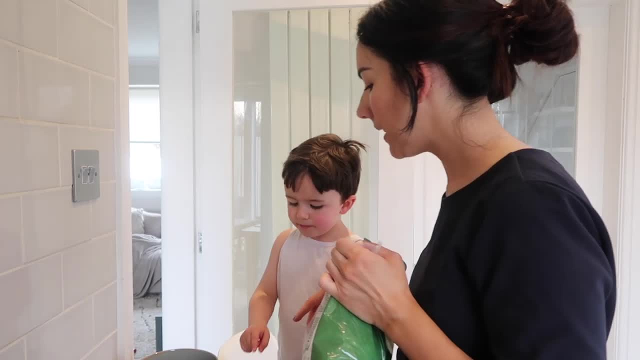 Cookies. So this is one of my favourite recipes. I absolutely love to make cookies, But this one is extra special because I love anything with cinnamon in it. So this one starts off with some porridge oats And we're just pouring them into the bowl. 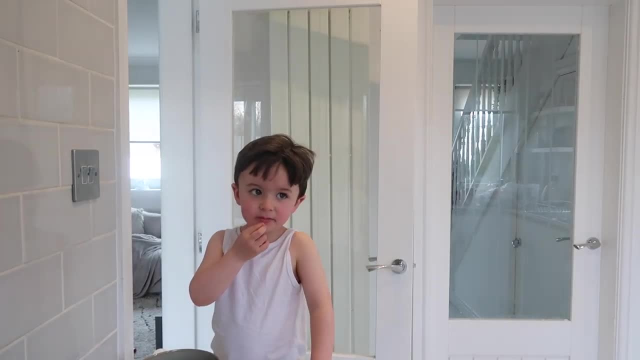 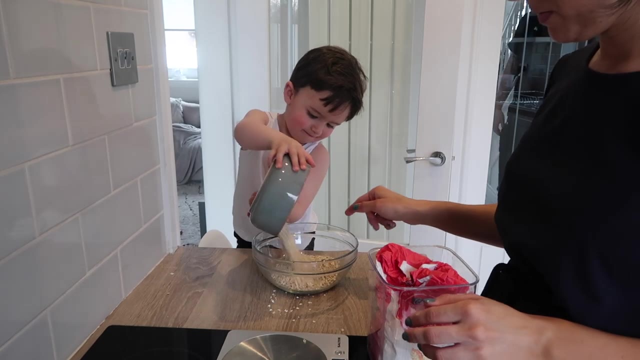 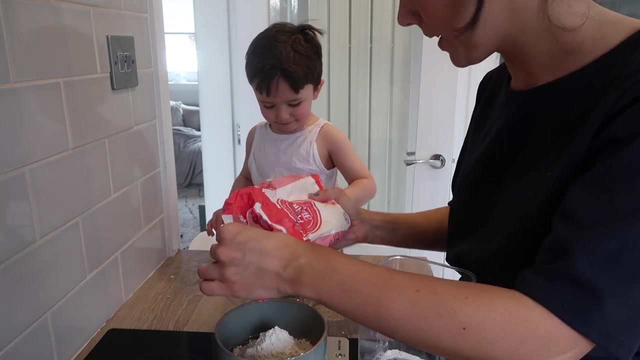 And you can always guarantee that when you're not looking, the toddler will try whatever is in there, even if it's just dry porridge oats, And then we're just adding in the flour and we're going to mix up. This is actually a really good one for kids because there's quite a lot of dry ingredients at the start. 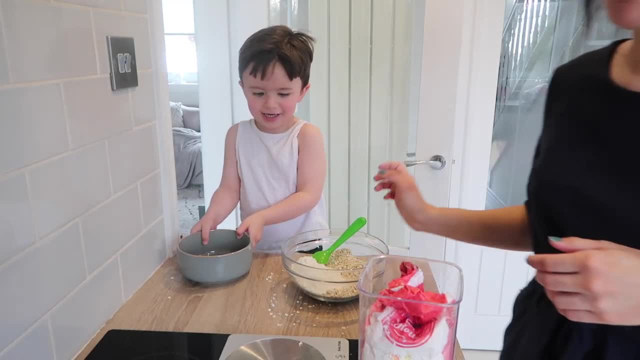 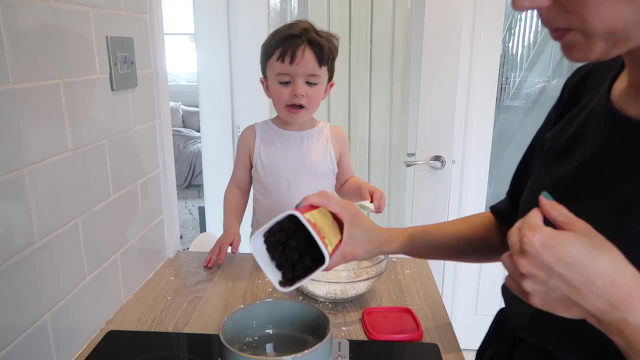 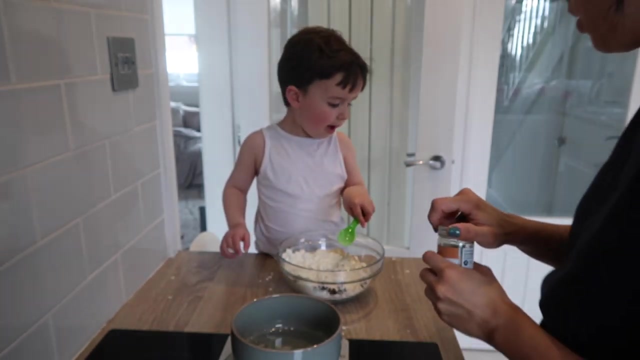 So they can just mix and mix and mix while you continue to add things in. So next we're going in with some raisins And, obviously, having a wee snack while we do that. Next we're adding some baking powder, Some cinnamon, which you can always add a little bit extra if you really like it, like I do. 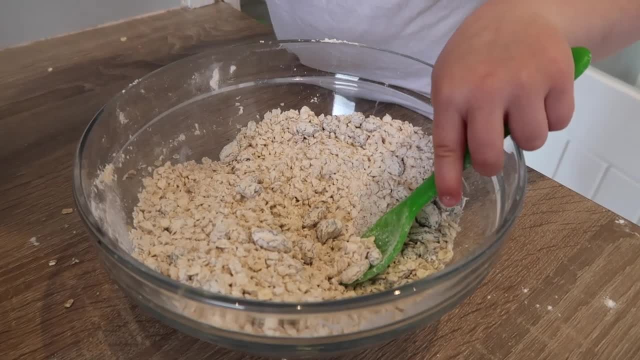 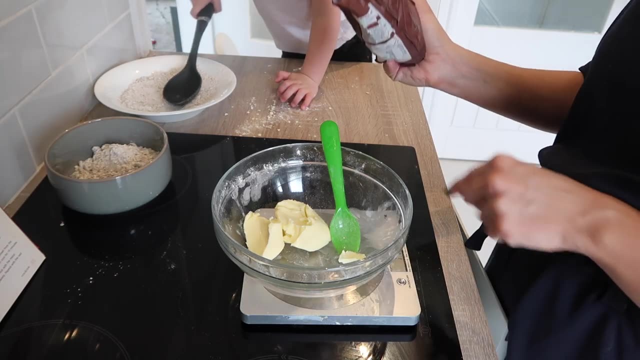 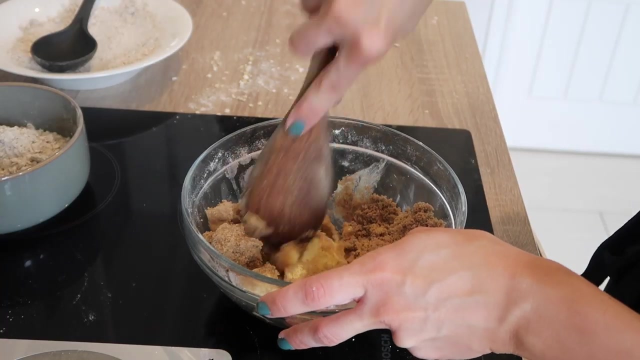 And then a few shakes of salt and just mix it up until everything is even. And then you want to just start in a separate bowl again and use your softened butter and sugar And then just combine them until it's even. You can tell. I don't really have any other phrases to use on baking videos. 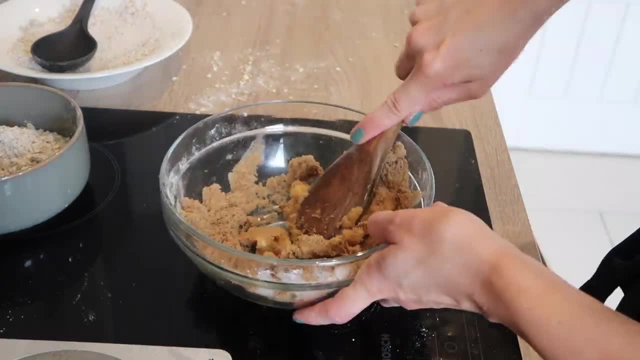 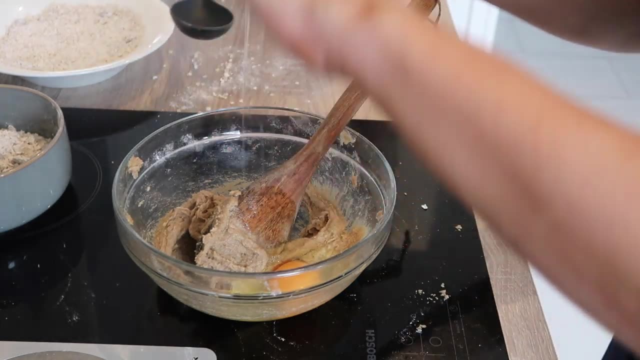 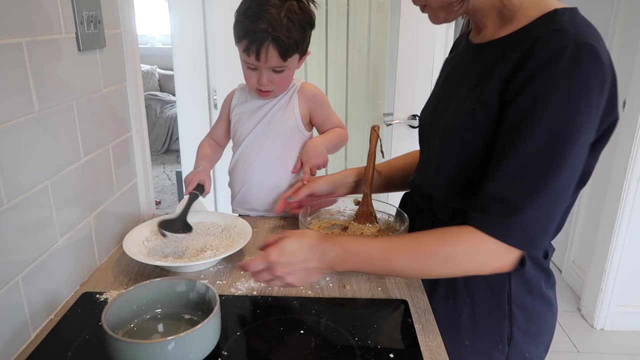 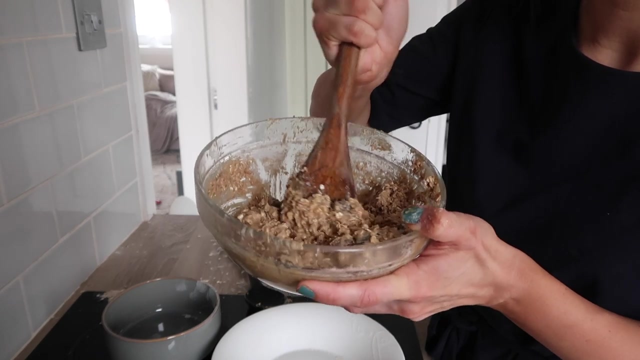 Sorry for repeating myself constantly. And then I'm just going to crack an egg straight into this bowl, Mix it all up, and then we will slowly add in our dry ingredients And then, once it looks like this, it is ready to go. It's a very, very firm mixture, so it's quite easy to put out onto the tray. 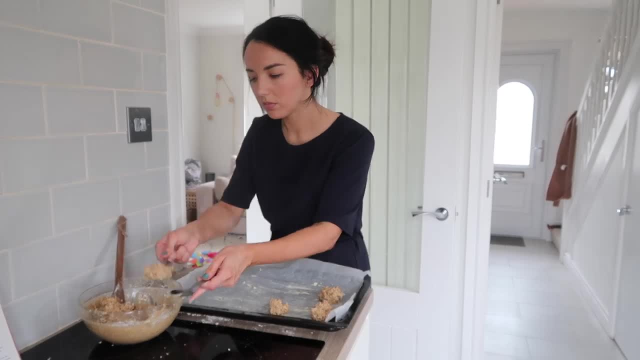 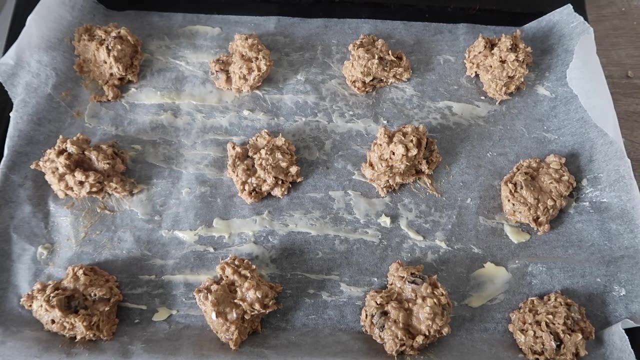 So you want to just put out a baking sheet onto your tray and then just spoon the mixture out. So try not to have them too close together because they do obviously expand as they cook. So I think I managed to get about 12 of these on the first tray. 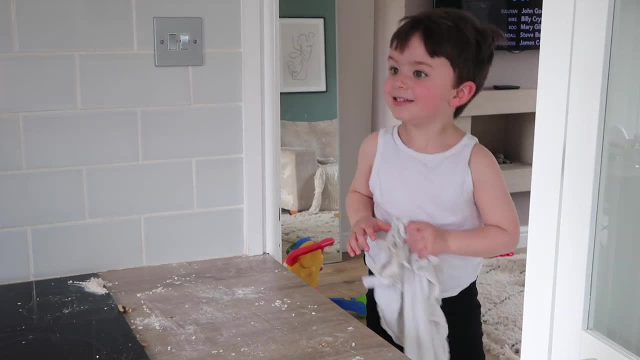 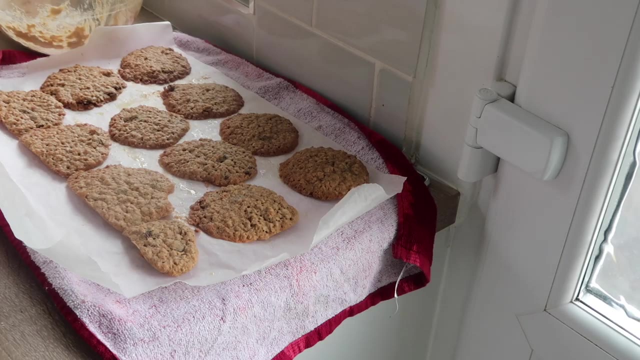 And then on the second tray we managed to do another 8 afterwards, So we did have quite a lot of biscuits to get through, But that was a welcome challenge, because these are amazing. They're so good, especially when they're straight out the oven. 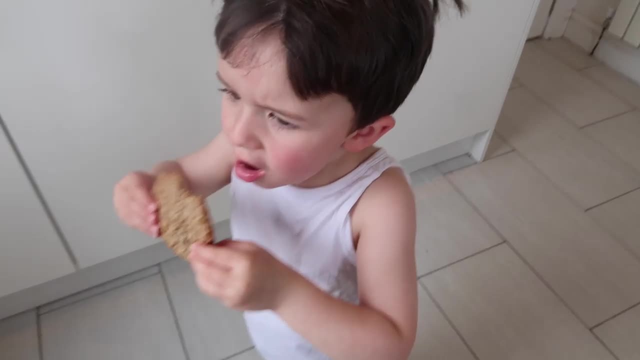 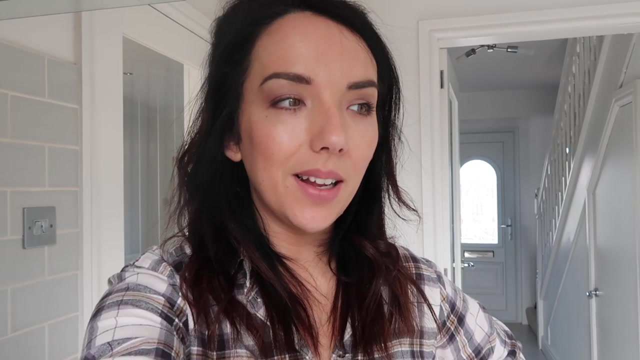 These are definitely a must try, and they're actually really easy to make. They are so so good. Okay, so today's recipe is one that I don't even think Oliver is going to join in on. This is going to be cinnamon swirls in the oven. 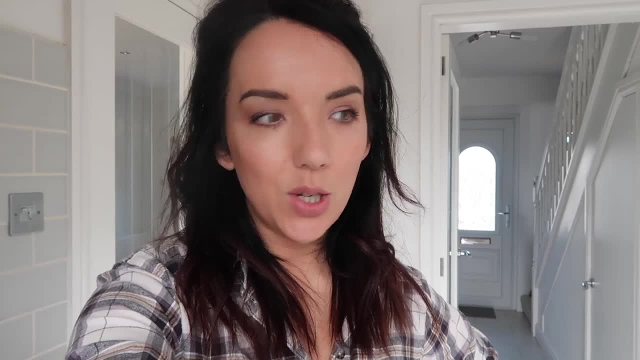 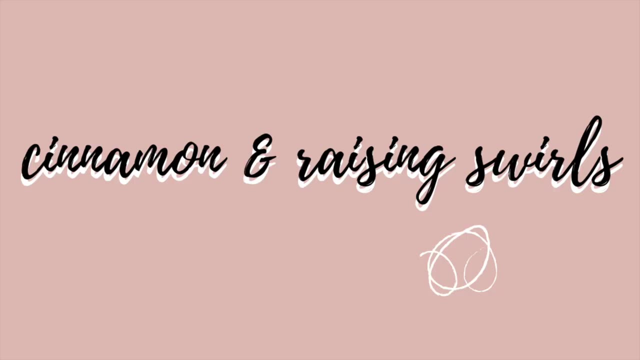 It's a very quick recipe but Oliver is watching the TV just now and doesn't want to join in. But I'm going to share it anyway because this is a really good one for kids, because it's very, very easy to do And I'm pretty sure he'll join us at some point. 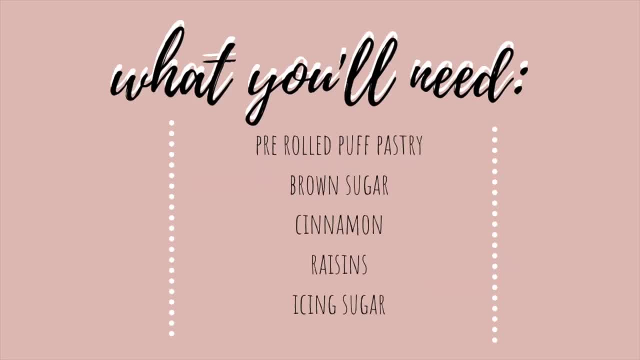 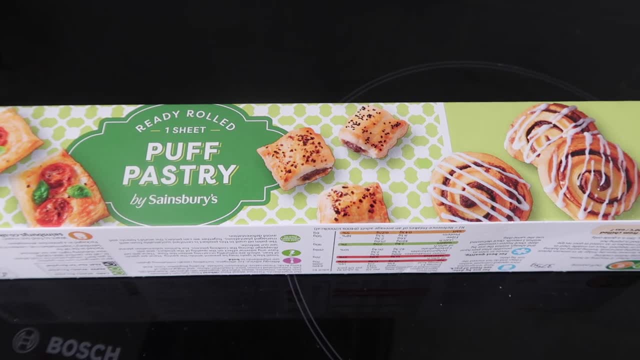 So this is a really good one to do in the morning, because they make a really good treat breakfast. For this you just need some rolled puff pastry And everything is really done for you now You're just really putting a topper on before it goes into the oven. 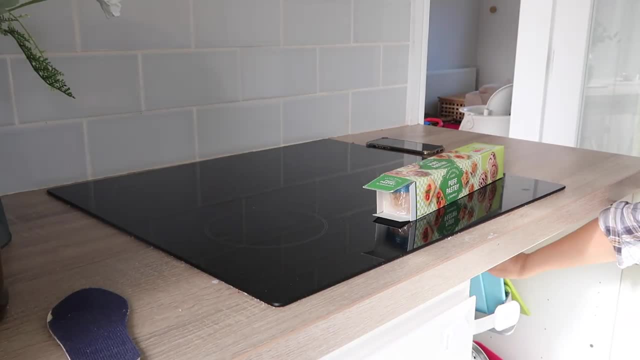 This is a kind of thing that we're making. So you just want to take the puff pastry out of the box, And I'm actually only going to cut off a little bit of this, because we definitely don't want to have loads and loads of pastries. 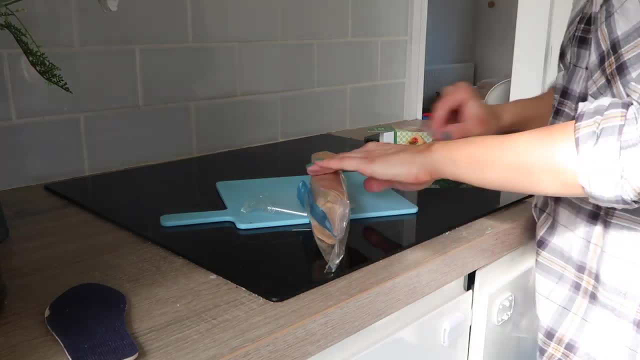 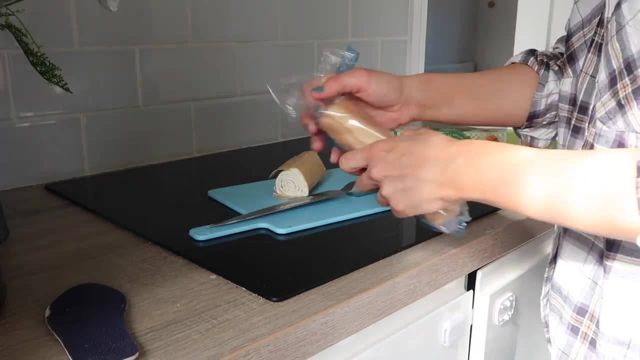 I just could not. I couldn't trust myself with them. The good thing about this is you can use this puff pastry for so many different things. Like you can put ham and cheese on it, You can have it for lunch time as well for them. 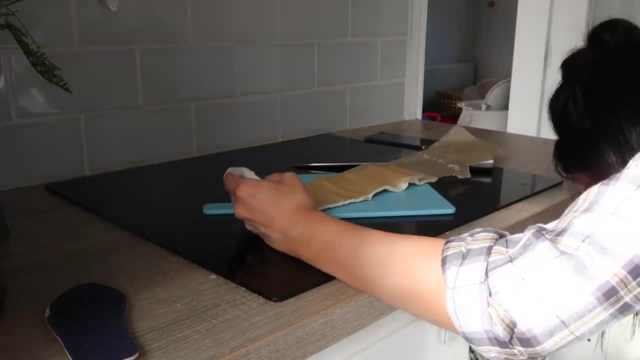 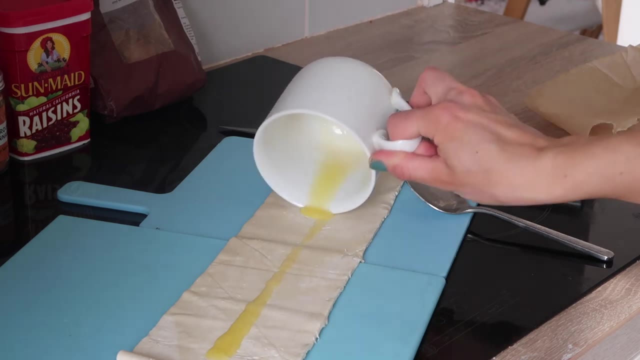 And this one made about 6 mini cinnamon swirls, So it was a good measurement for it. So I think that was about a third of it. So all you want to do is just add some melted butter over the top just to coat the pastry. 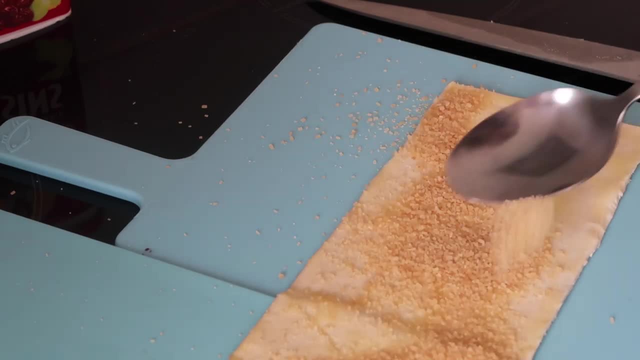 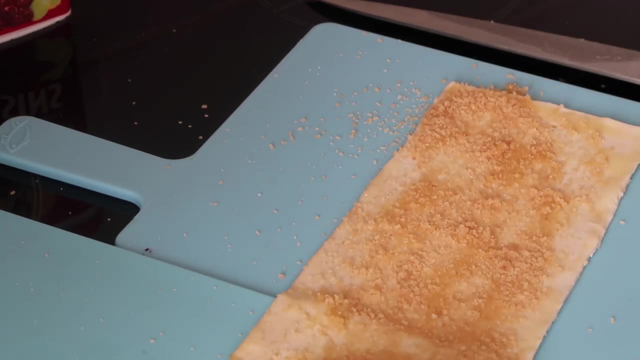 And then, over the top, we are just going to sprinkle some brown sugar all over. You can see, this is not the healthiest of recipes, But it's a wee treat and it's so, so good. So once we've covered it all in sugar, we are going to add our cinnamon over the top as well. 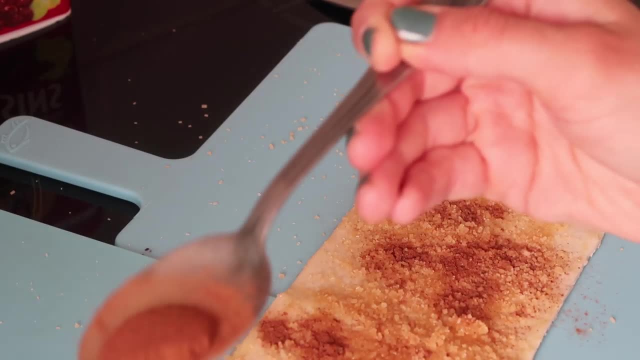 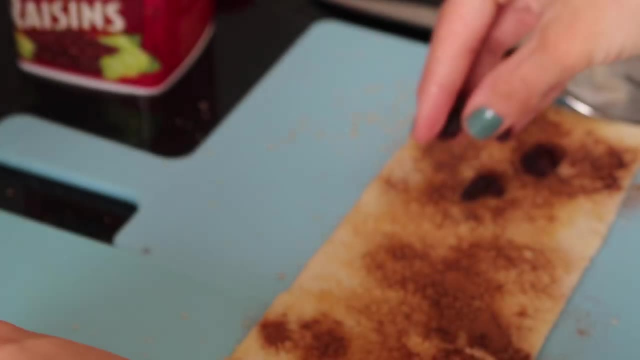 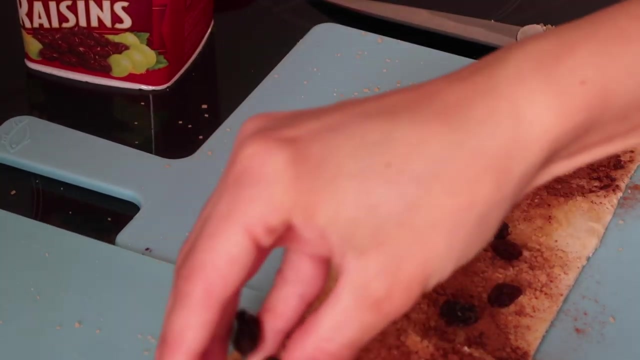 So again, just put on as much as you want. There's no measurements for this one, Just freestyle it. And then I'm also adding in some raisins as well, because I think raisins that come out of the oven are amazing. I'm not into them dry, but when they're heated up they are my favourite thing ever. 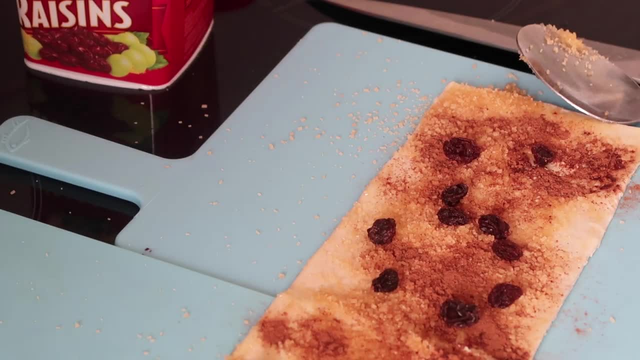 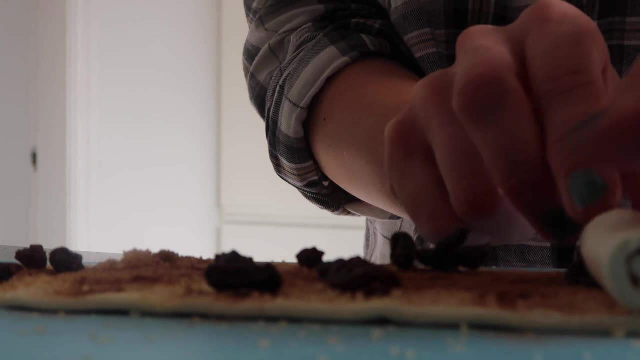 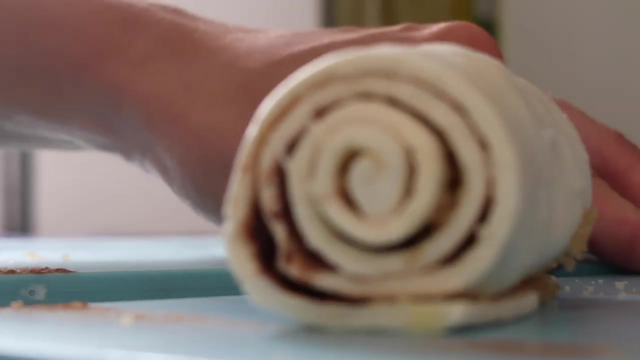 Especially with cinnamon. Does anyone else agree? And then all you want to do is just get rolling, Roll your full pastry up from one side to the other, And then you're just going to cut them into slices Again. if you take your time and cut them really nicely, then you will get a really nice shape. 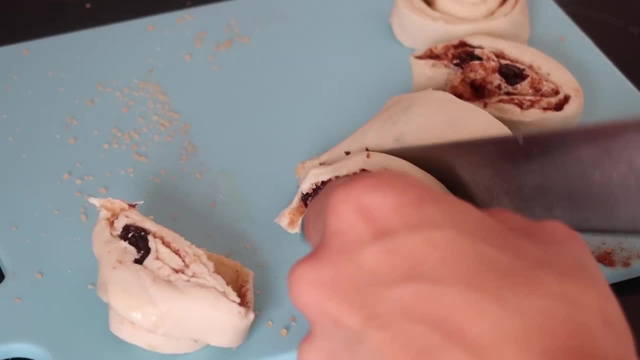 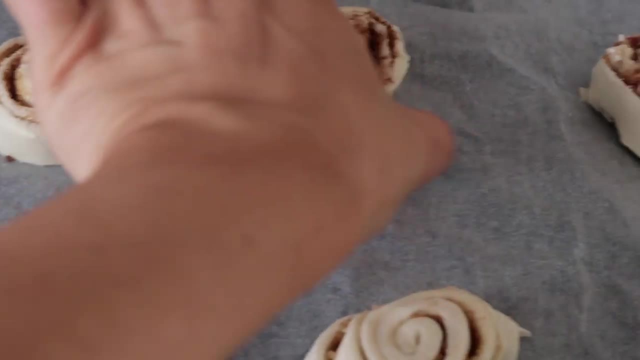 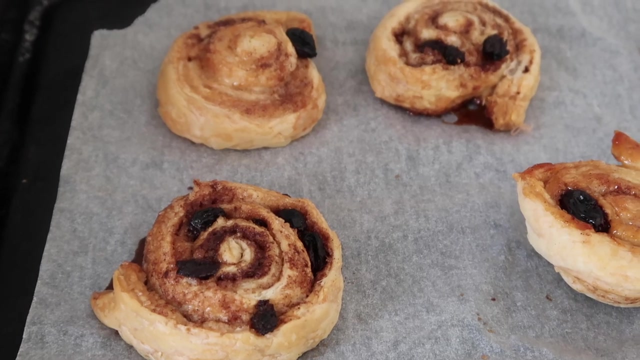 Or if you just go for it, then they still taste as good as the ones that look nice. So line them up on greaseproof paper And pop them in the oven at 200 degrees for 20 minutes. I can't even tell you how good these smell. 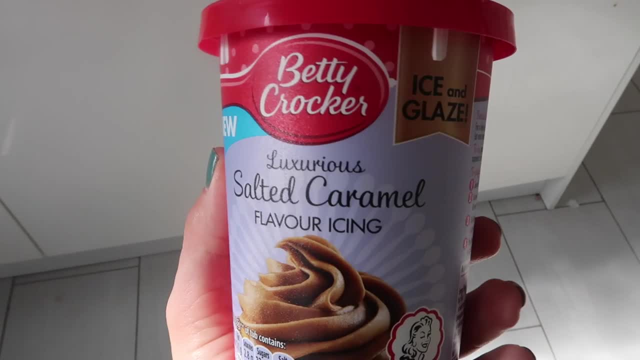 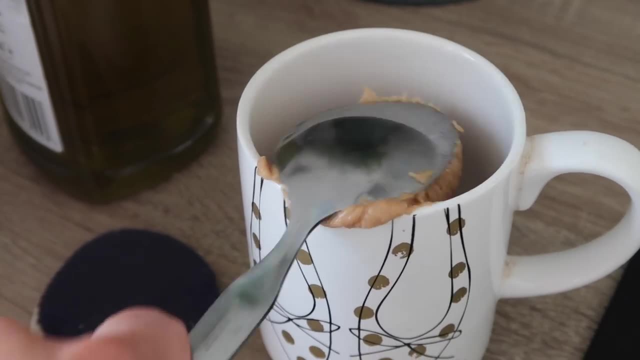 They're absolutely amazing, And we're just going to use the leftover of this salted caramel flavour icing. We're just going to pop some into the microwave now, just to show another way of using this. This is such a good thing if you're planning on doing lots of baking during lockdown. 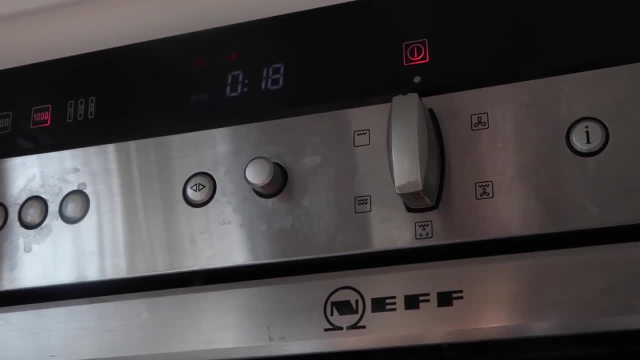 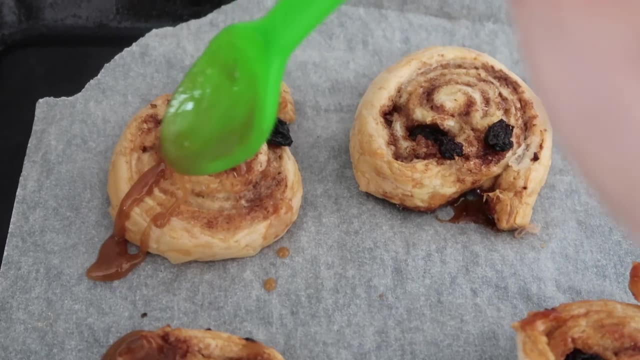 So I just put it in for like 20 seconds And it melts it into melted icing. I'm so bad at doing voiceovers, I apologise, So I'm just going to drizzle this over the top And it just makes them even more delicious.